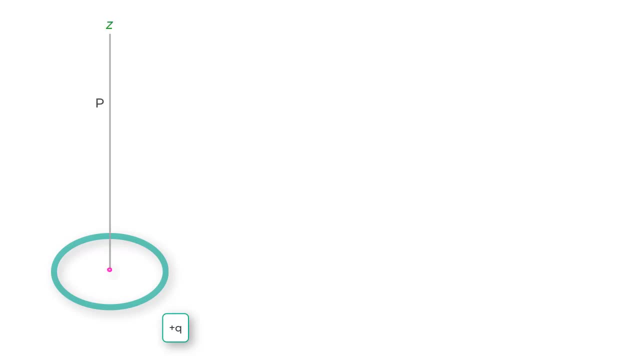 at a point, P above it, and let's say P lies on the z-axis. Now, what is important here is that you try to understand how we are approaching this problem, because if you do so, you will be able to apply this method to other patterns of line charges, like an arc or a straight line, as well. 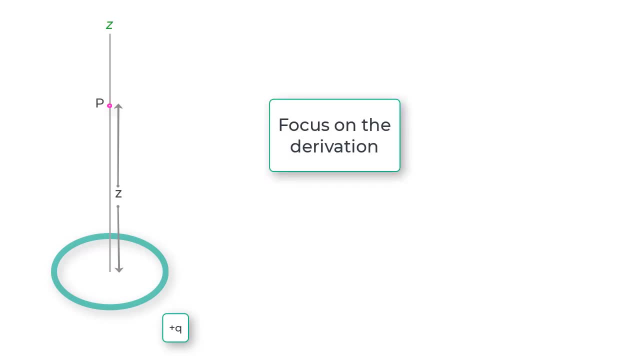 So focus more on the derivation than the final answer and when you get to the final answer, try to interpret the results in various ways. what will give you a better depth of understanding of the topic. So a good start could be that we pick a very, very small element of length ds here and say: 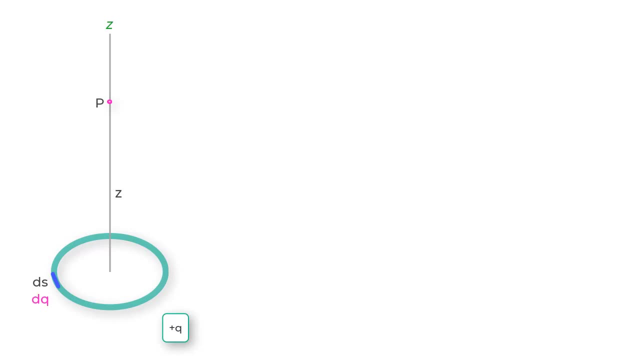 the charge on it is dq and constraint. ds is very small, dq should also be very small. Then we can say that the charge per unit length is nothing but dq divided by ds, and let us term this as lambda, or dq is equal to lambda times ds. Now this charge elements. what you see here is: 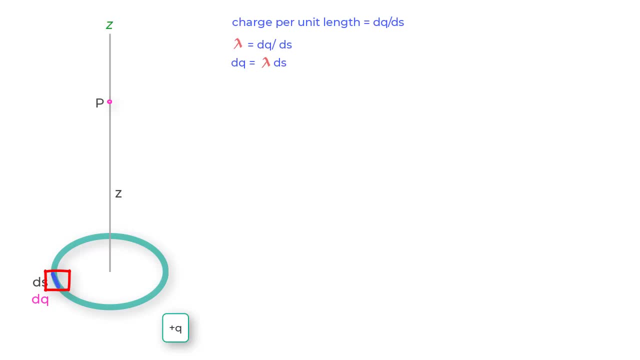 going to set up a certain electric field at P that is, at a distance r from the element, and we can say that this small value of e set up here is de, and this de should equal one upon four pi. epsilon dq upon r square, which again can be written as 1 upon 4 pi. epsilon lambda, DS upon R. 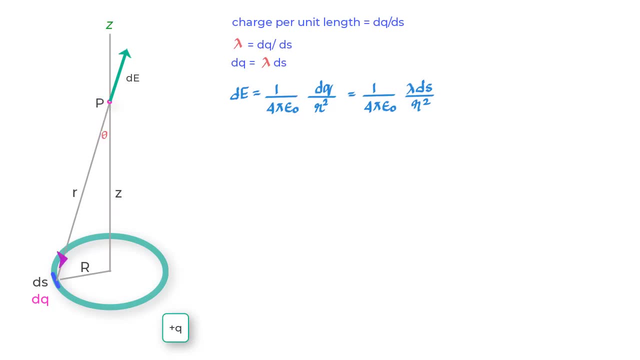 square, but then, this being a right angle triangle, R square should equal Z square plus R square. so we can substitute the value of R square as this in the equation to get: the: e is equal to 1 upon 4 pi, epsilon lambda, DS upon Z square. 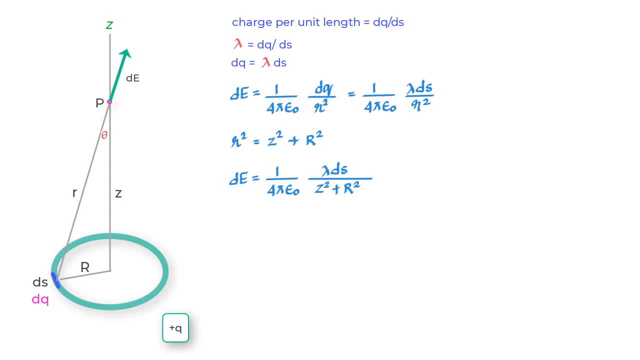 plus capital R square. now you see that we are lucky here, that every ds element through the length of the circle is at the same distance from point P and would therefore contribute the same value of de at P, which is this. so it makes our calculations a little easier, and we'll see that as we move forward. so let us 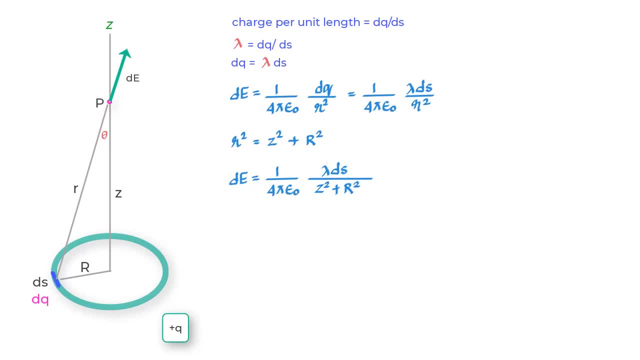 now take an element of ds, right opposite this one, and we can say that the line from this element also to P there should lean at an angle. theta and the direction of electric field would be this: now, if you take the vertical components of both these vectors, you will see that they point in upward direction. but if you 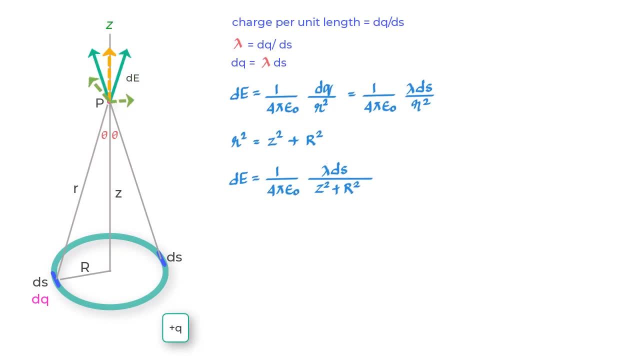 take the horizontal component of each of these vectors, you will see their project out in opposite directions and therefore cancel each other. and you would see that, by symmetry, any ds element you take on this circle, we'll have its horizontal component of electric field cancelled by an equivalent ds element right opposite it. so what you end up having is only the. 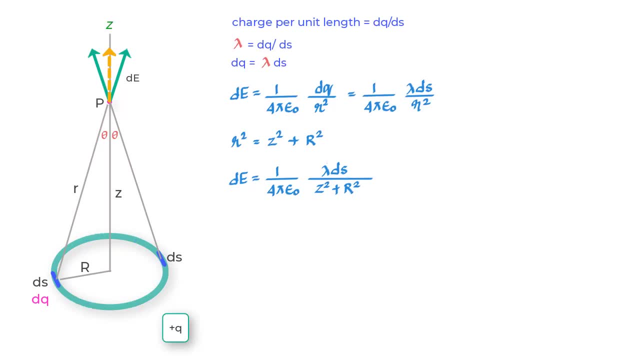 worry of this sign if h s will rise when I place density and this vector here is not looking straight. in other words, the vector is not these vectors because whatever we going to get from these vectors, vertical components as the net electric field at this point, due to each element ds on this ring. 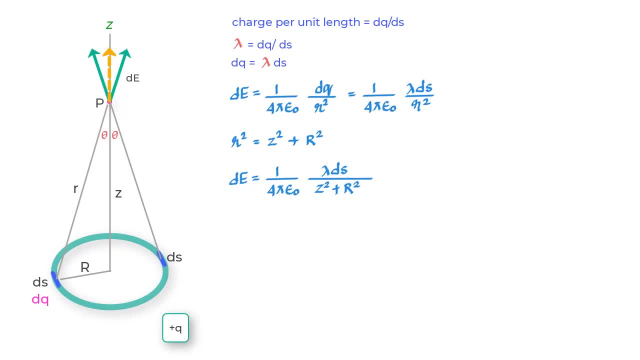 so this also makes things easier for us. and further, all the vertical components are in positive z direction, so you could say that's also good. now the question is: how can we add up all the vertical components of the electric field by each element ds on this ring, and what you'll see is: 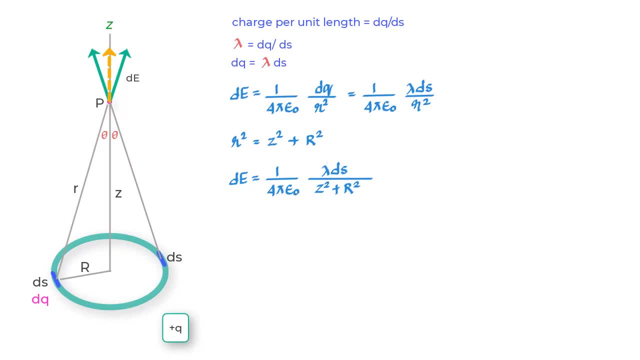 that integral calculus can help us in doing this submission. so the value of the vertical component is nothing but d e cos theta, and if we take cos theta is equal to Z upon R, we get cos theta equals Z upon R, which equals Z upon r, z squared plus r squared under root. So we can write dE cos theta as equal to 1 upon 4 pi epsilon. 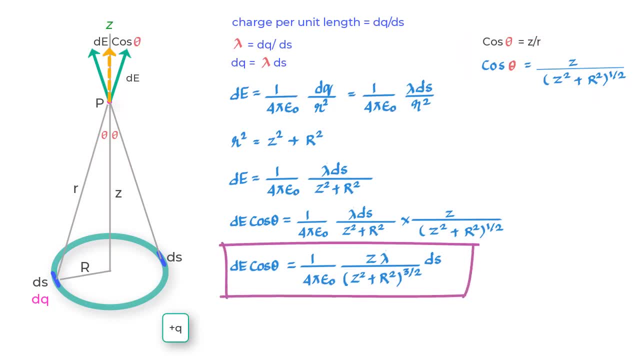 z lambda upon z squared plus r squared to the power 3 by 2 dS, And using integral calculus, we sum up the contribution of each dS by integrating them from S starting at 0 all the way to S is equal to 2 pi r. So what we're doing here is using integral calculus. 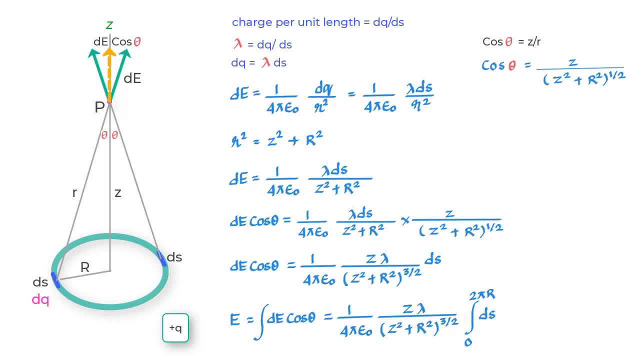 to account for the electric field due to all charge elements, dq on the ring and summing them up, So we say that the total electric field is integral of dE, cos, theta, which is equal to z lambda upon 4 pi epsilon, z squared plus r squared to the power, 3 by 2. 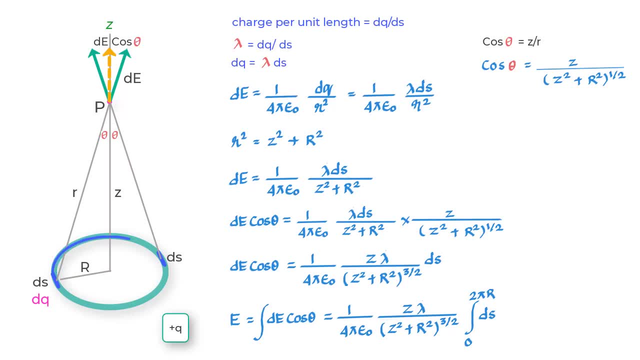 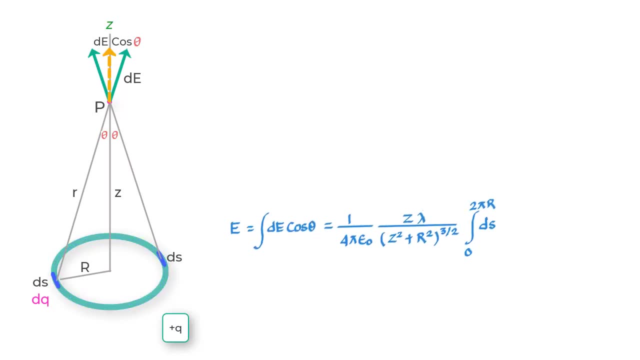 integral of dS as it changes from 0 to 2 pi r. Now, if you integrate this, what you get is this expression. But then we can say that lambda can also be written as total charge on the ring divided by the total length. So lambda can also be written as q upon 2 pi r, because you see 2. 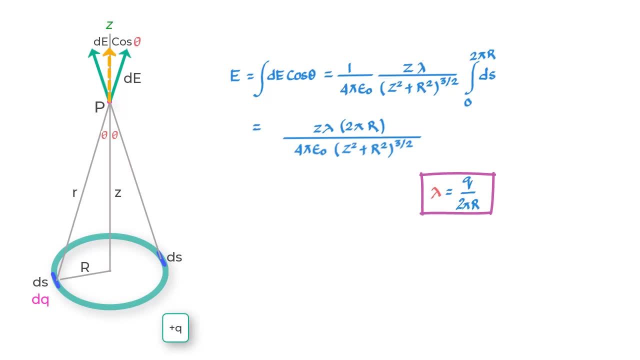 pi r is a circumference of this ring and Q is the, the total charge on the ring. and if we substitute this value in this equation, what we get is this expression. so you can see that we have taken Q as a positive charge on the ring to do the 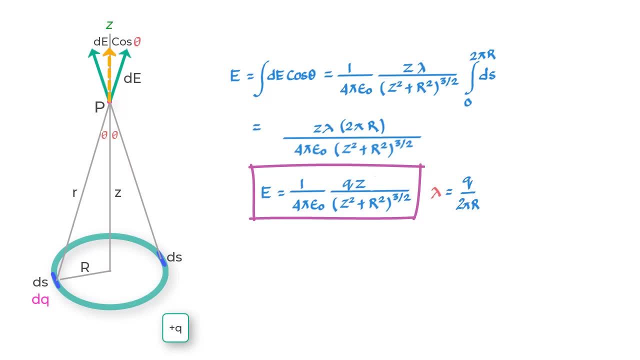 derivation. but if we take it as a negative charge, E value would become negative, indicating that the direction of the field is downwards towards the ring instead of upwards, that it is with a positive Q charge. well, we could do some interesting checks with the formula we've just derived to see if it is. 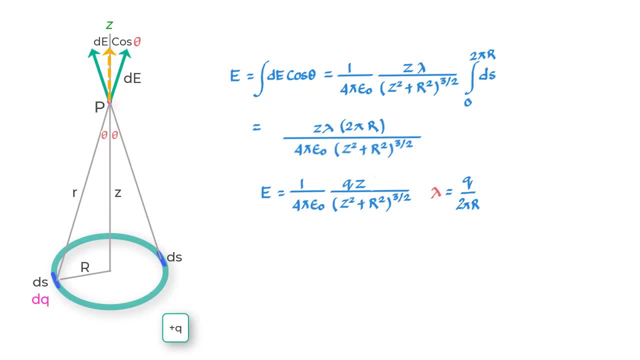 really correct. so let us say that Z is much greater than R, such that the square of Z would be a lot higher than square of R. so we can go ahead and drop the R square value and approximate Z square plus R square as Z square only, and then what we get is: E is equal to 1 upon 4, pi, epsilon Q upon Z square, and